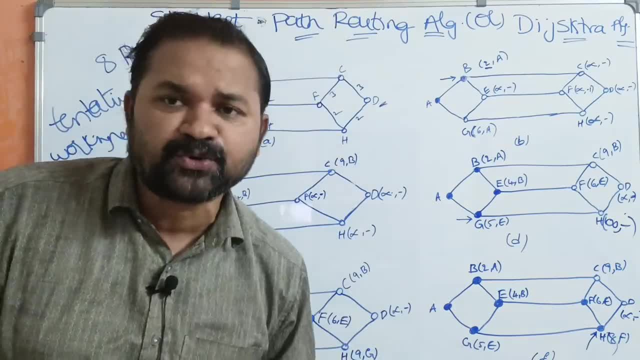 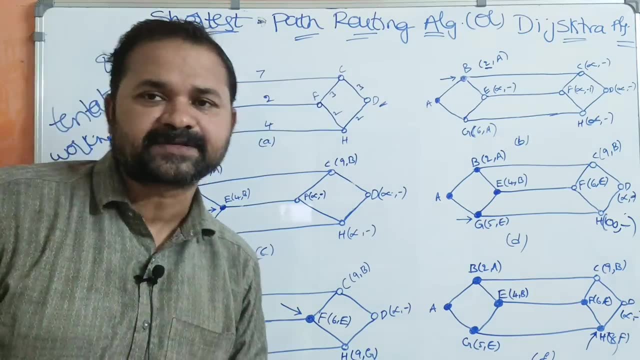 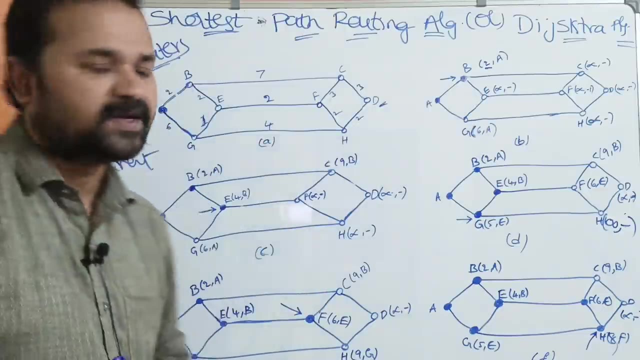 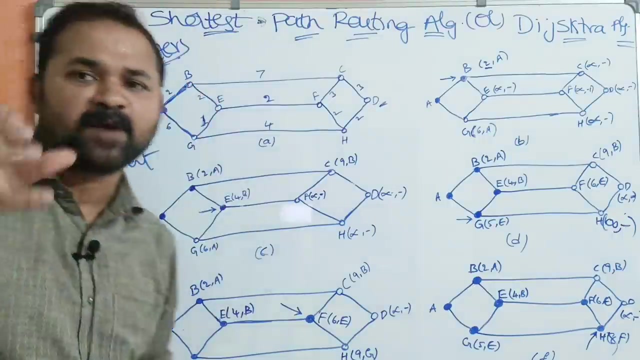 the shortest path from source router to destination router. Here we have a graph. This graph totally contains 8 routers: A, B, C, D, E, F, G, H. Here the routers are represented by nodes. Here the nodes are A, B, C, D, E, F, G, H, So this edge represents that communication. 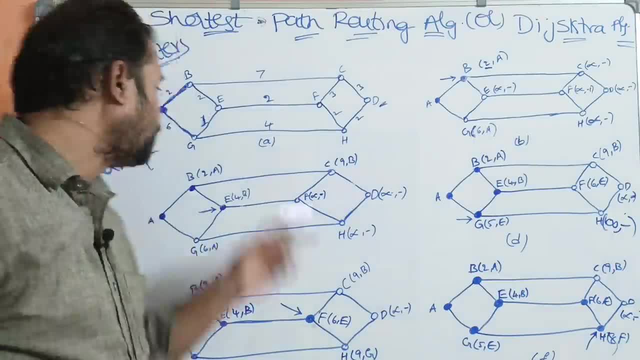 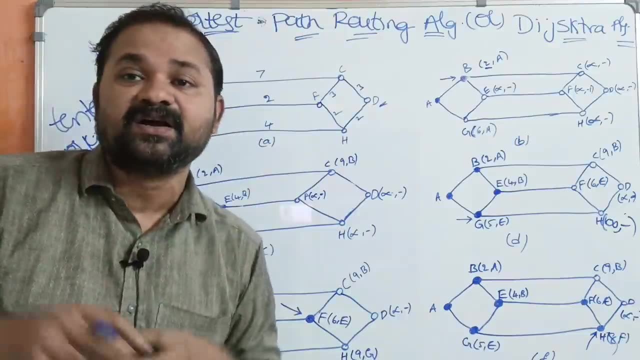 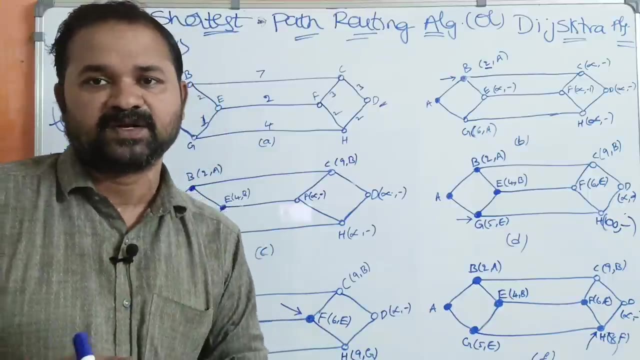 link. So what is the distance from A to B Or what is the distance from E to F? So this number represents distance or cost or weight, or we can also call it as delay also. So here we have, here our major aim is we need to 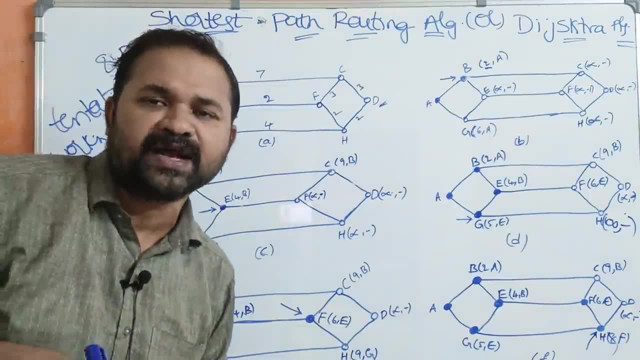 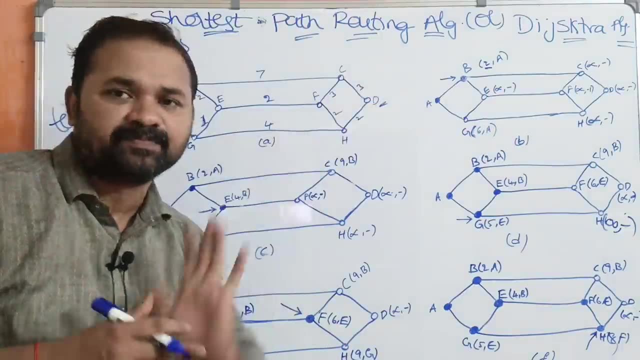 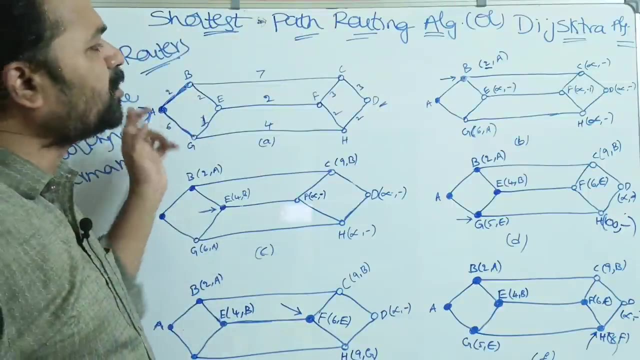 find out the shortest path from source router to the destination router. So let us assume that source router is A, destination router is D, So we have to find out the shortest path from source router to destination router. So we have to find out the shortest path from source A- A node- to the destination D node. 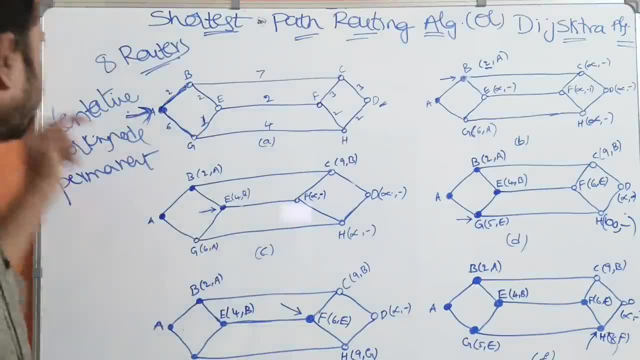 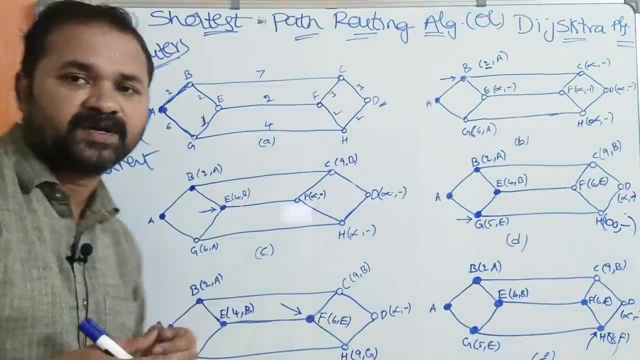 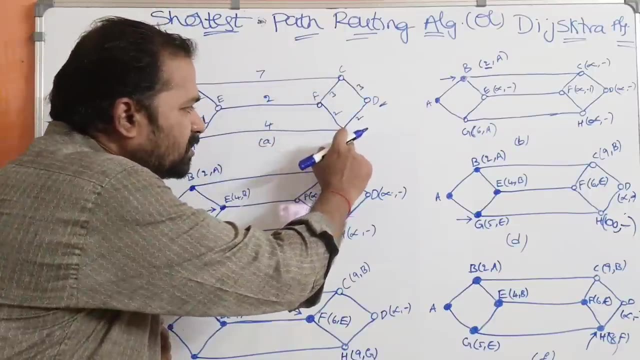 Okay, Here we have three types of nodes. The first node is tentative node. Second node is working node. Third node is permanent node. So tentative node means it is a wide circle. So C is a tentative node, D is a tentative node. So this wide circle is nothing but tentative node. 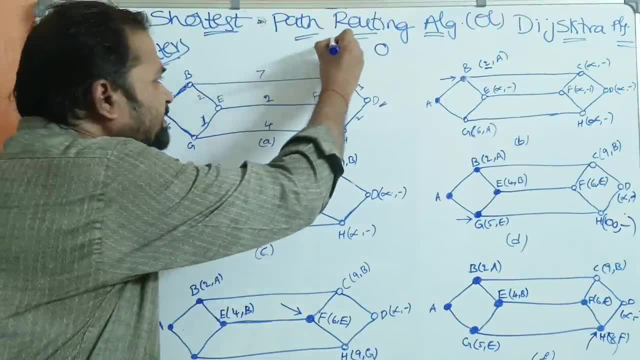 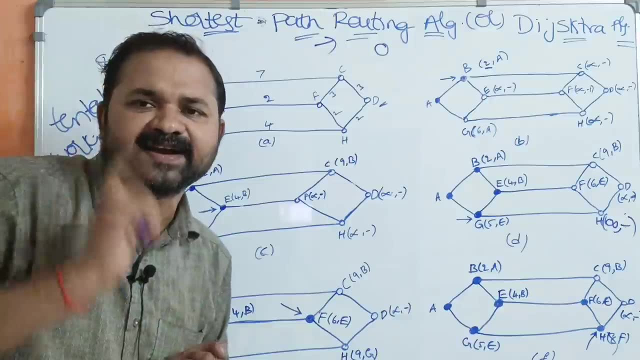 Because current working node means it is represented by arrow, So before the circle we have some arrow symbol. So if you observe, here in every graph we have one current working node. So here A is the current working node In this graph, B is the current working node In this: 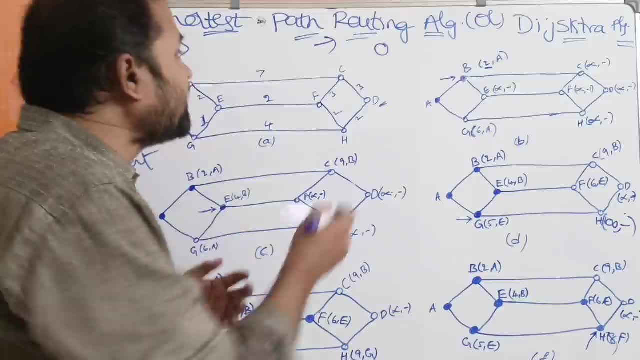 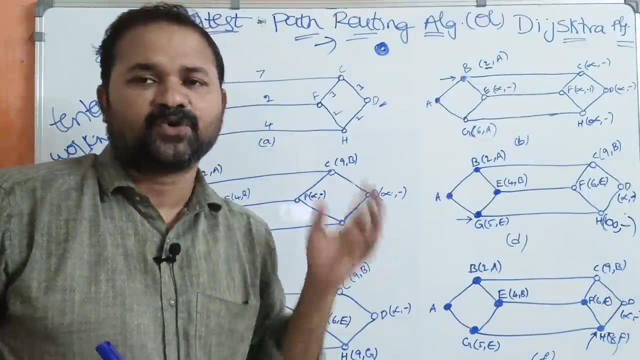 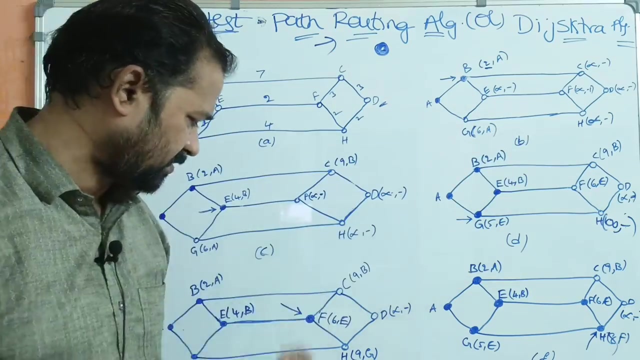 graph G is the current working node. Likewise, And the permanent node is represented by a solid circle. Permanent node is represented by solid circle. So here we have. we have to solve this problem. We have, for that we have. we have. we have one, two, three, four, six steps. So let us see step 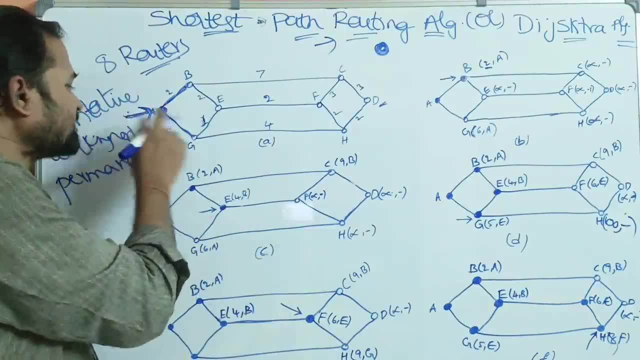 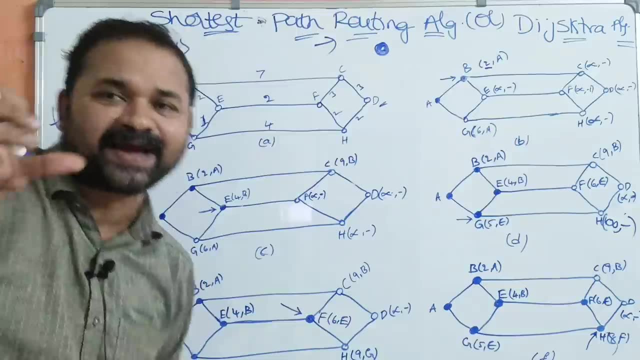 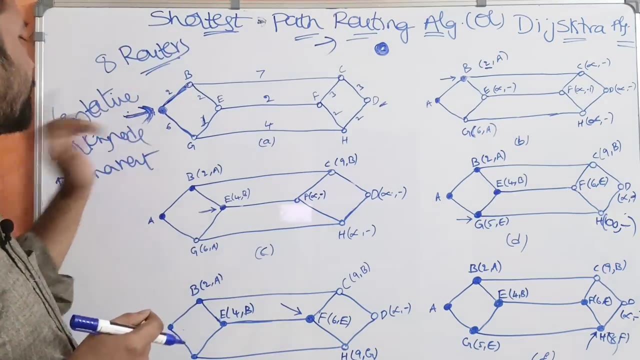 by step. Initially we have to assume the source vertex as the current working node, So that is represented by arrow, And we have to make the first node, that is, source node, as the permanent node, Source node as the permanent node, Okay, And remaining all nodes are tentative nodes. So 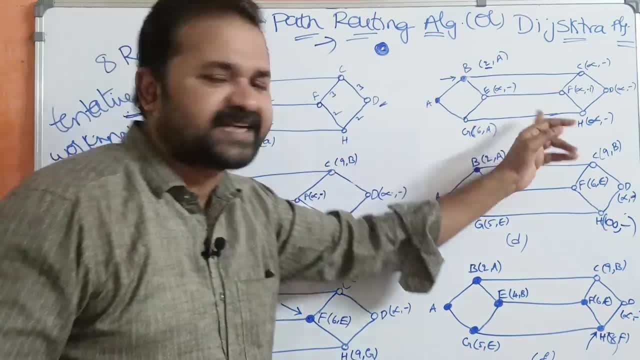 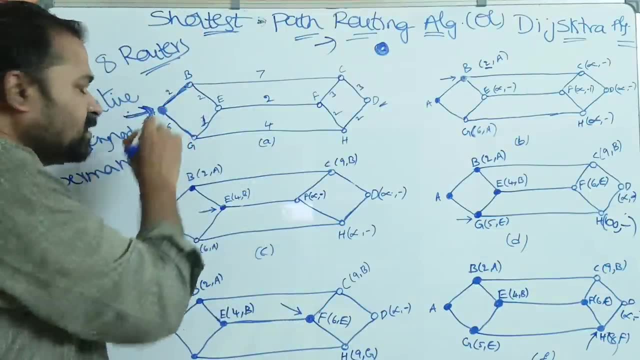 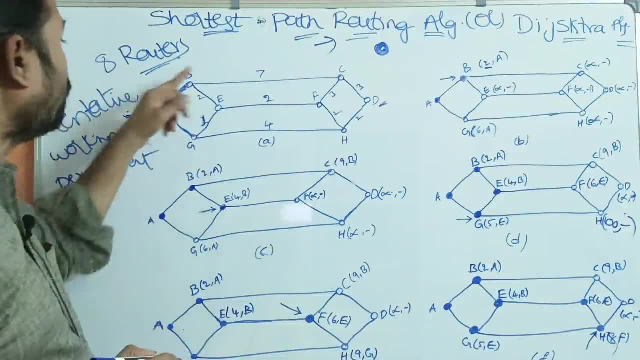 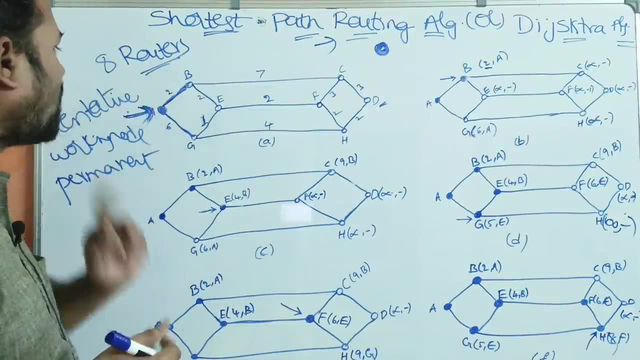 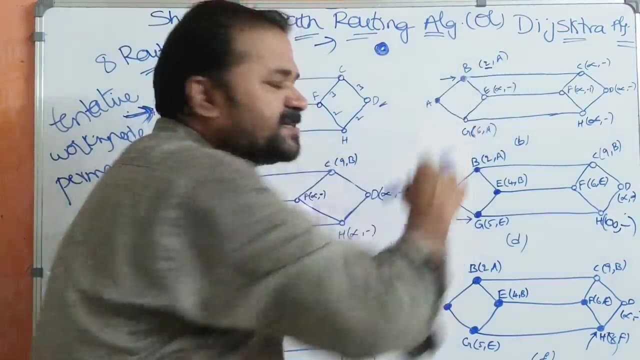 the neighboring routers of A. So the neighboring routers of A are B and G Here. what is the cost of B in order to traverse from A to B? The cost is 2.. So here we we can update this path length by a pair. The first argument represents the cost. 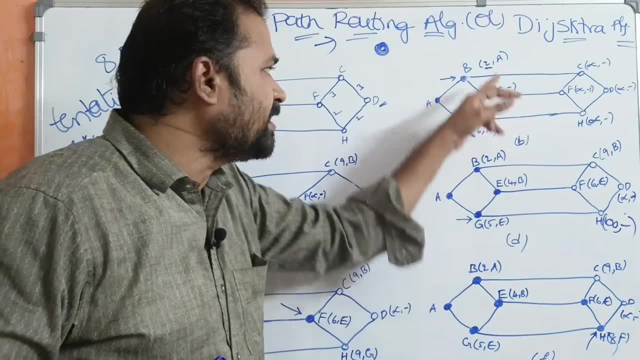 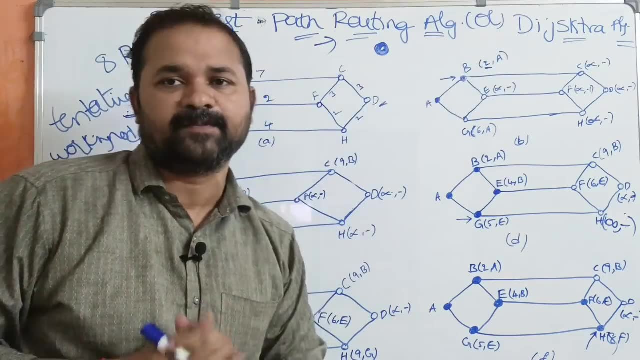 Second argument represents the current working node. So here the cost is 2, the current working node is A. So we are traversing to B from A. So 2, A. Next, what is the cost of G? That is 6.. 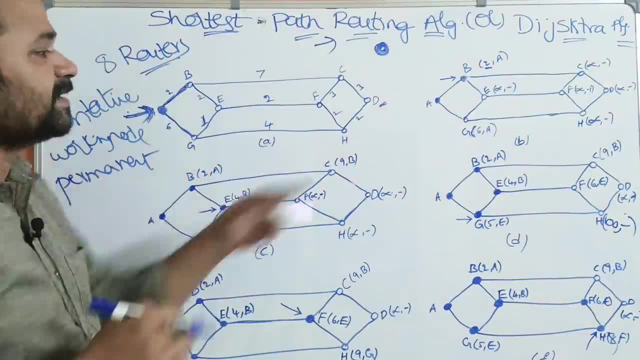 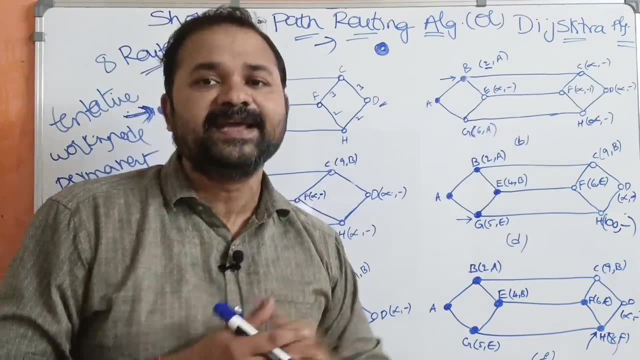 So this cost, this length, is updated by 6, A, 6, A. Next, we don't know E path length, F path length, C path length, H path length, D path length, So that's why they are updated with infinity. 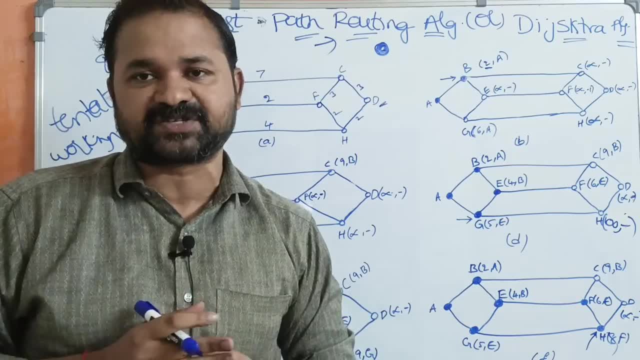 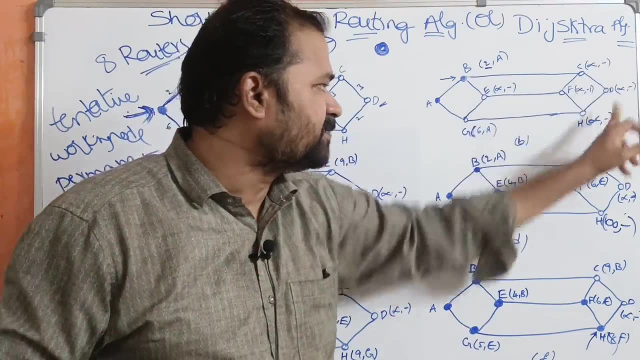 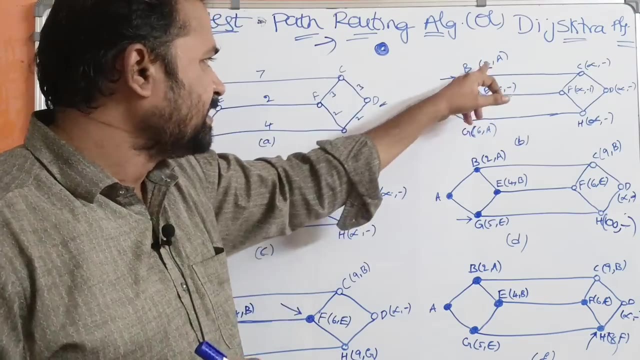 Infinity specifies that we don't know that. path length cost. Minus specifies the current working node is not known to us. So minus specifies: this hyphen specifies: current working node is not known. Next, here we have two, two paths. Here the cost is 2, here the distance. 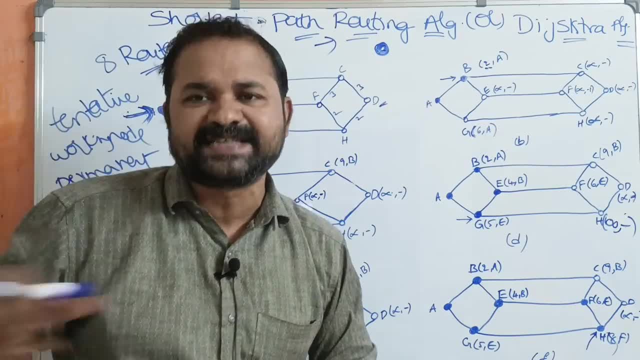 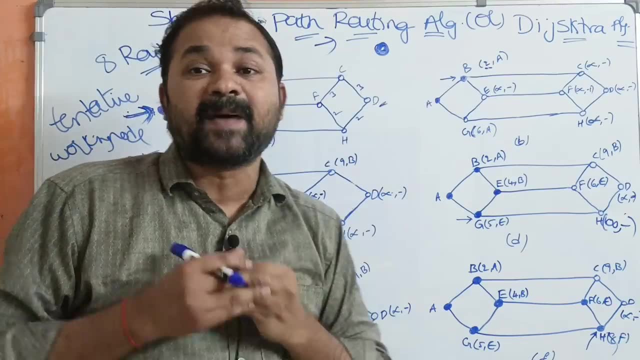 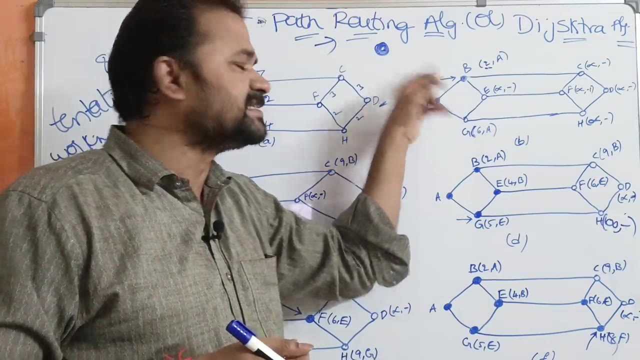 is 2,. here the distance is 6.. Out of 2 and 6,, 2 is the smaller value. So we have to make permanent node. So permanent node means solid circle, So this arrow represents this is the current working node. So in the next step, what we have to do, We have to explore B. 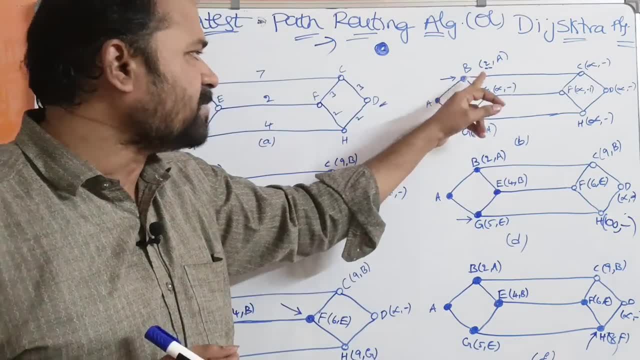 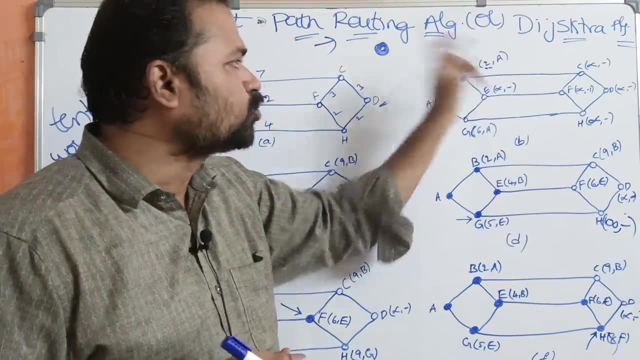 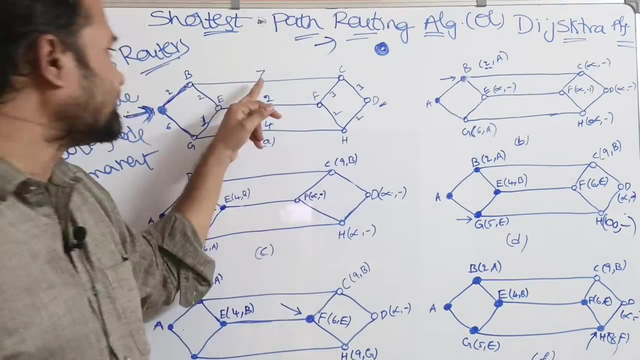 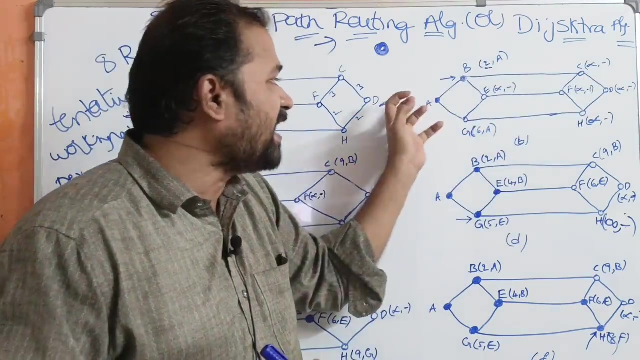 So find the neighboring routers of B. So the neighboring routers of B are E and C. Let us focus on C Here. what is the cost of B? 2. Let us find out the cost of C. Here the cost from B to C is 7.. So 7 plus 2 means 9.. So 9 comma hyphen. So here, here we are finding the path. 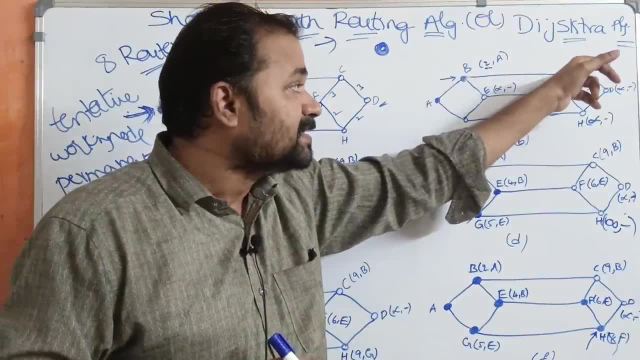 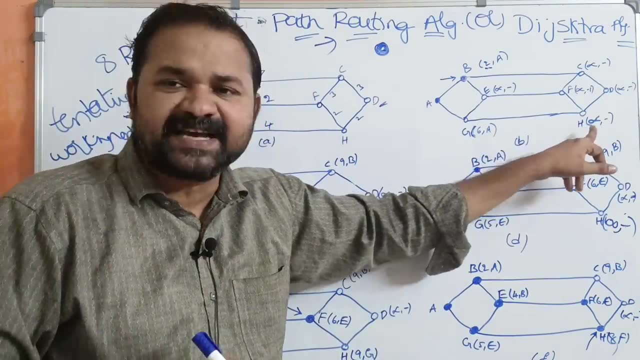 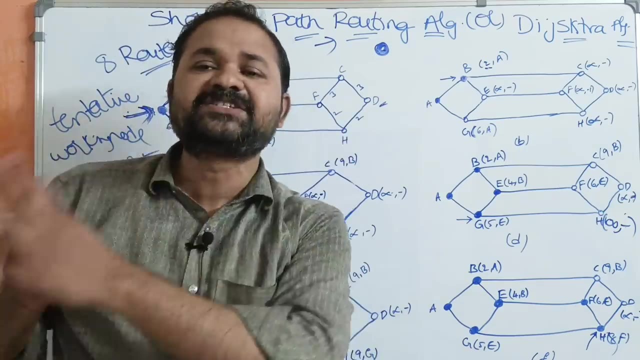 length of A, B, C. So here C, C distance means the path length from A to C. So likewise, H distance means the path length from A to H. Why? Because here our target is from source to destination vertex. we need to find the distance. 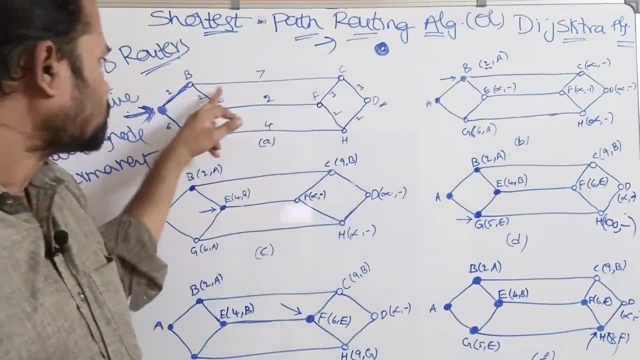 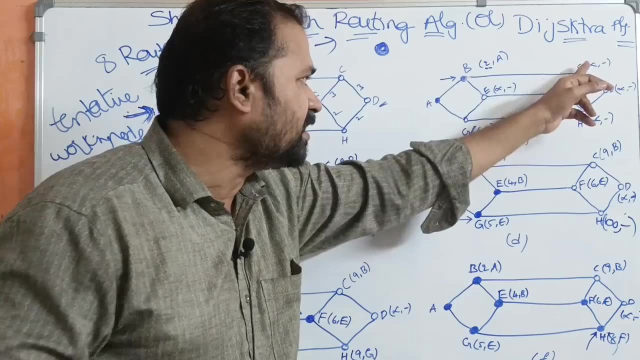 So here we have to update with here already the cost is 2.. So here this path length is 7.. So 2 plus 7 means 9., 9 comma, what is the current working? node B? So here we have to. 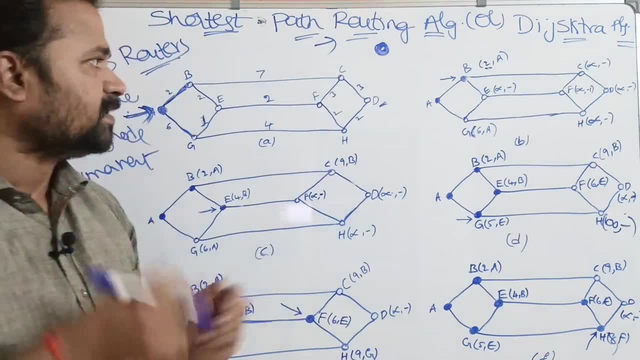 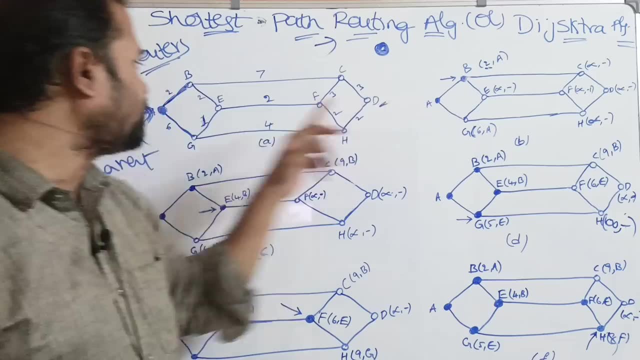 update C path length by 9, comma B. Next, what is another neighboring node E? So here the cost is 2, whereas the distance from B to E is 2.. So 2 plus 2 means 4.. So this path. 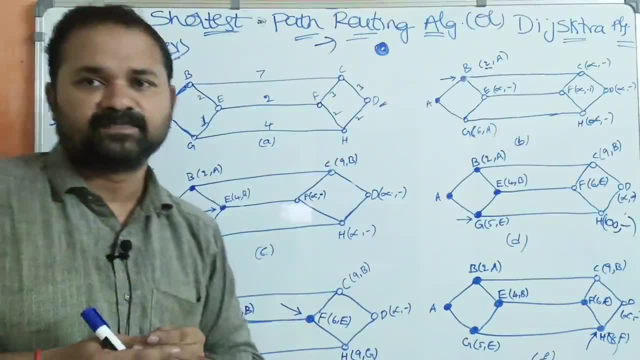 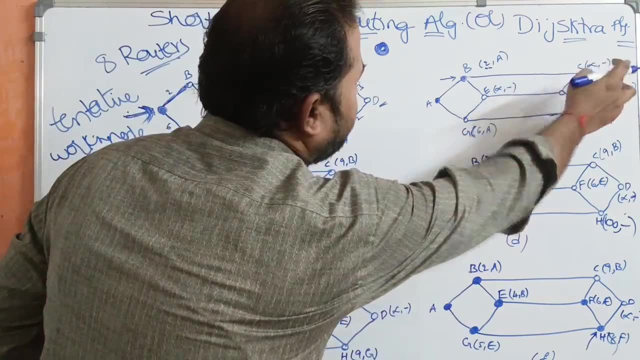 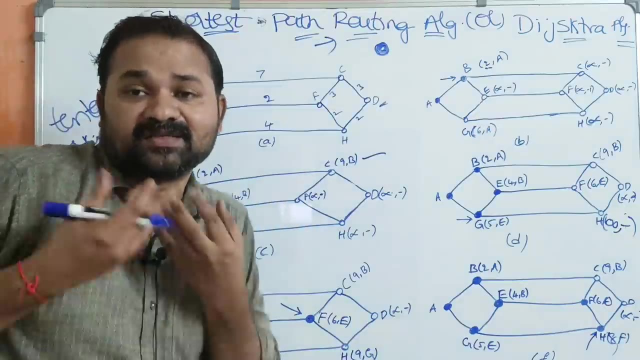 length is updated by 4 comma B, 4 comma B. So now, out of out of so here, what are the additional nodes we got here? Yeah, C node, Next E node. So out of 4 and 9, the smaller value is 4.. So we have to make this E node. 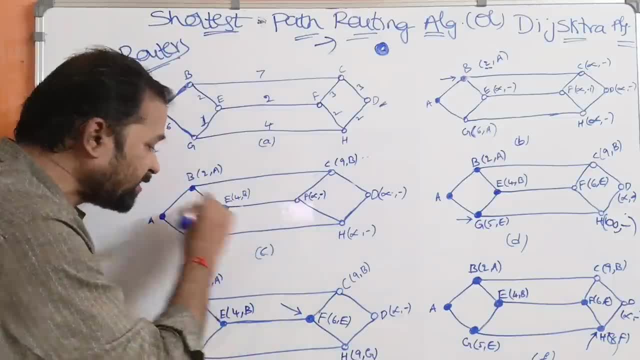 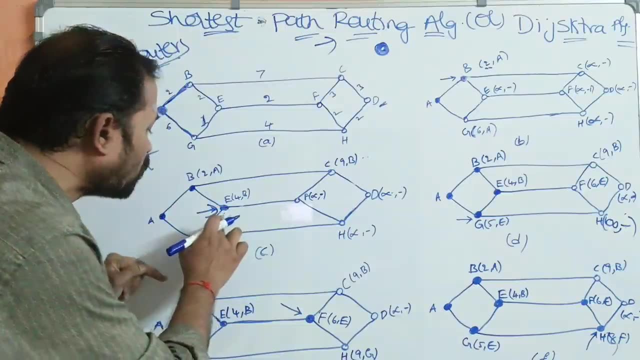 as the permanent node, This E node as the permanent node. So now let us explore E. Let us explore E. So what are the neighboring nodes? So we have nodes of E. We have two neighboring nodes, F and 6. F and G Already the cost. 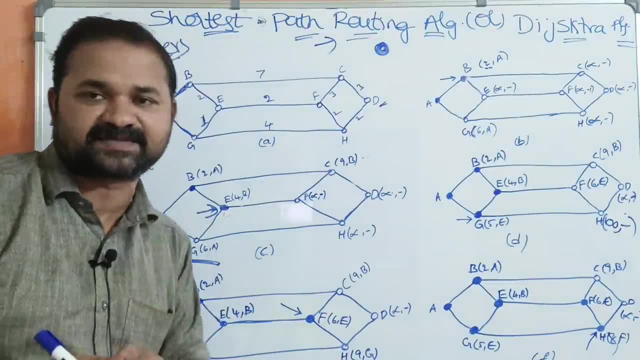 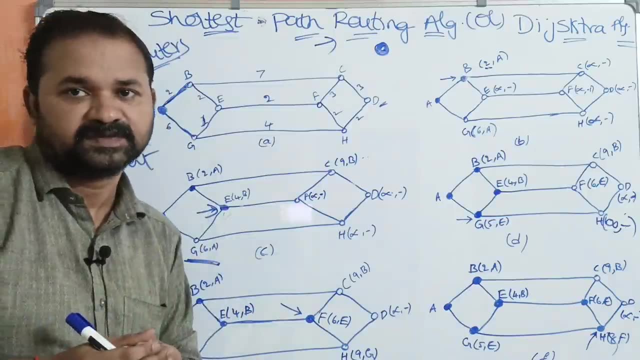 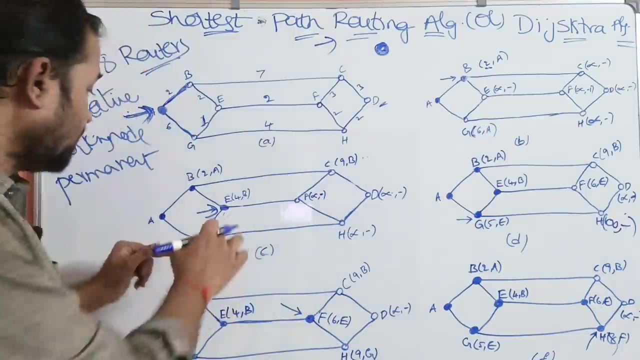 of the path length of G is already calculated, That is, 6.. Suppose, if we get a new value then we have to update with that new value. Why? Because here our major intention is always we need to find the shortest path length. If we focus on this one here, the cost of 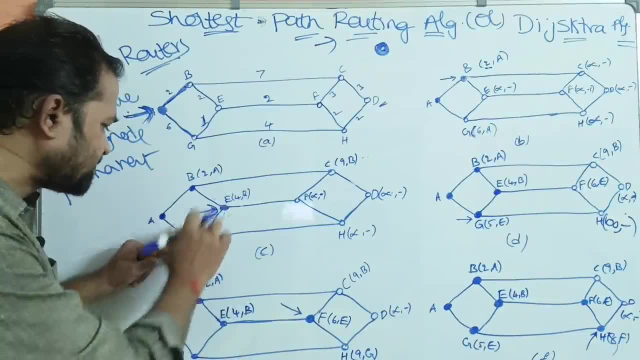 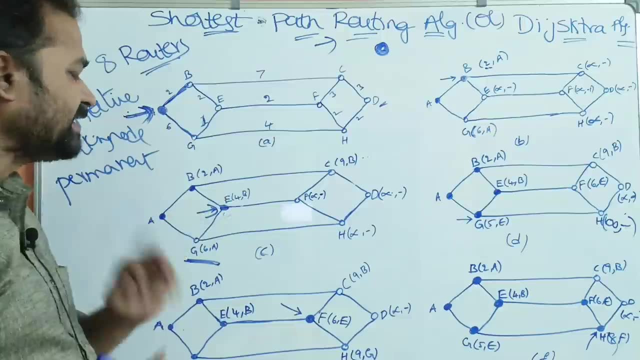 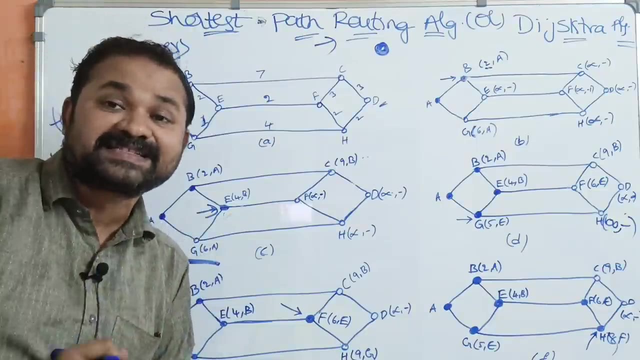 E is 4.. Next, the distance from e to g. the distance from e to g is 1, so 4 plus 1 means 5, so 5 comma e. so here previously we have 6, but now we got 5. 5 is less than 6, so we have to update the 6 by 5.. 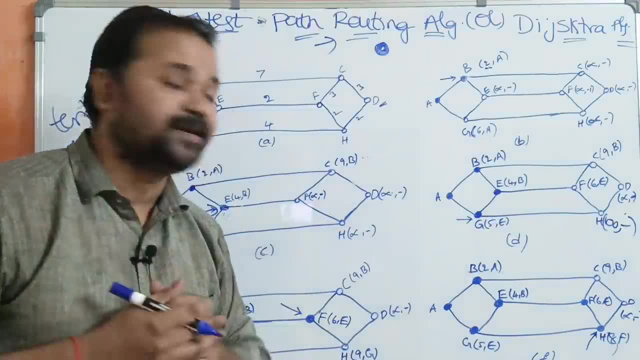 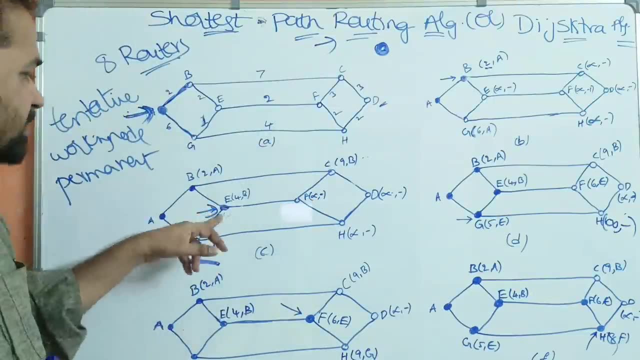 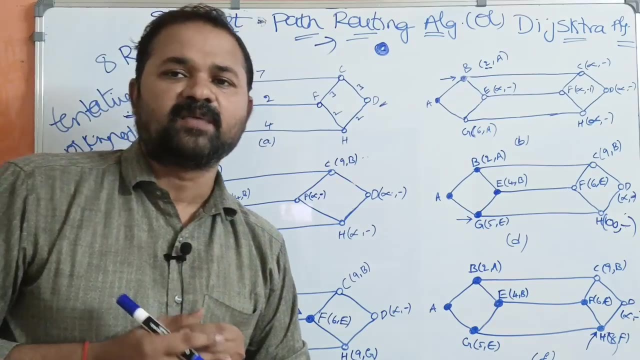 what is the current working node? from e? so 5 comma e, 5 comma e. next another neighboring node is f. what is the distance from e to f? 2? so 2 plus 4, that is 6, 6 comma e, 6 comma e. so now what are the? 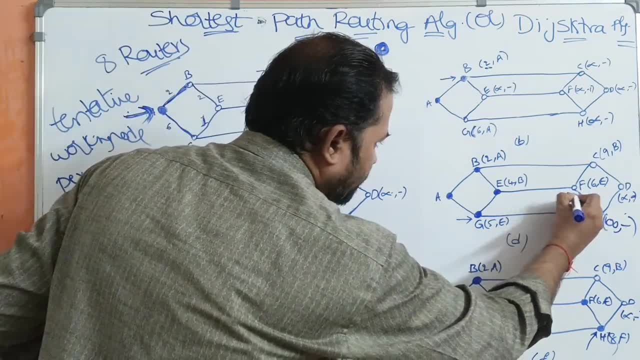 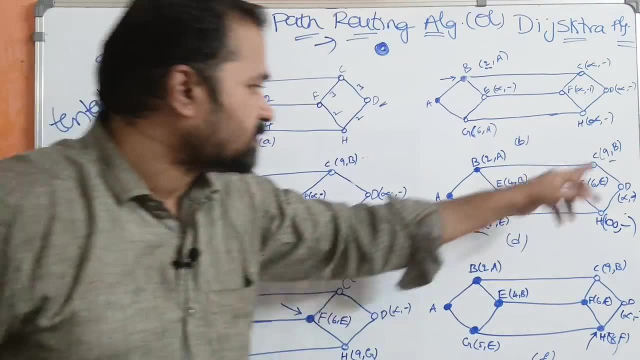 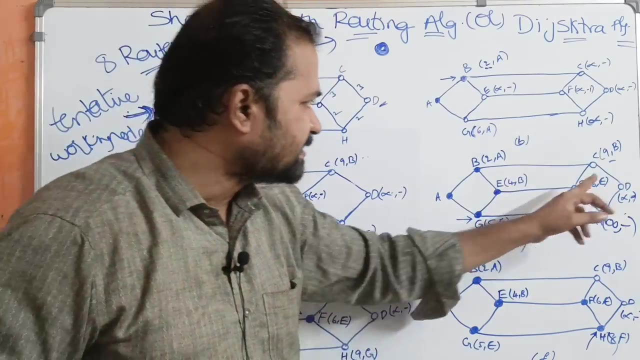 tentative nodes now. now here we have so f as well as g, f, g, and we have c also. so these are the tentative nodes. okay, yeah, out of c, f and g, 5, 6 and 9, which is is the smaller value, so phi is the smaller value, so we have to make this. 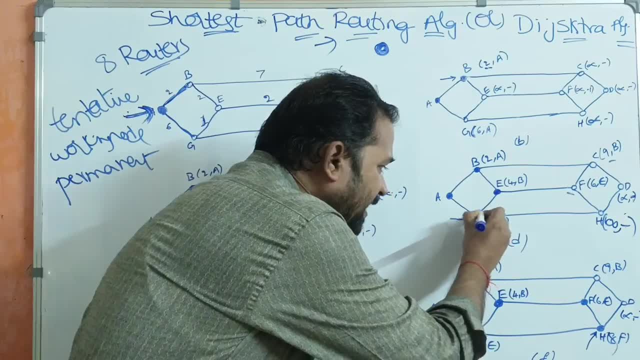 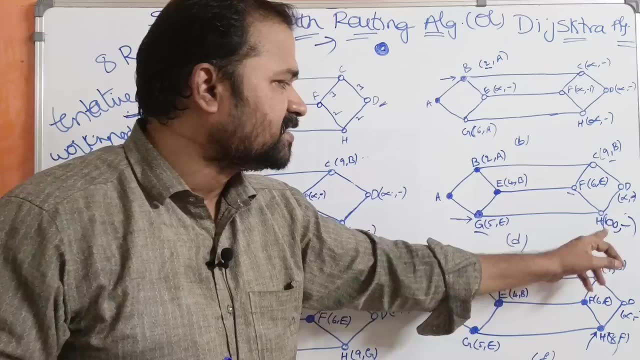 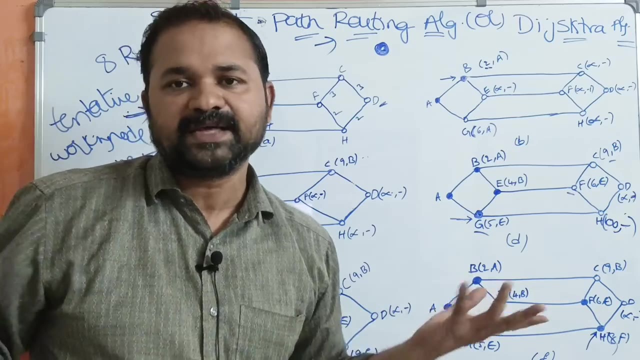 node as the current working node and made this node as the permanent node. so in the next step here we don't know the remaining paths lengths, so that's why they are updated by infinity comma minus only. if you don't know that path length- distance, then their path length is infinity comma minus. so in the next step 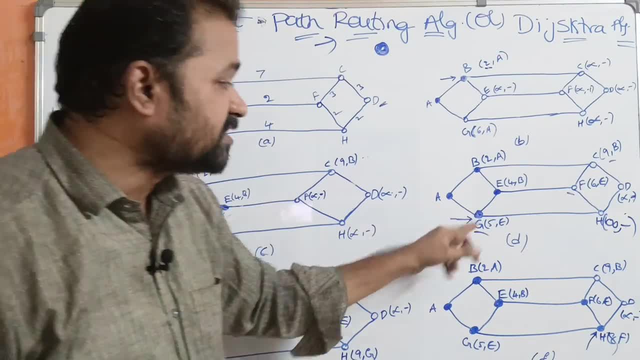 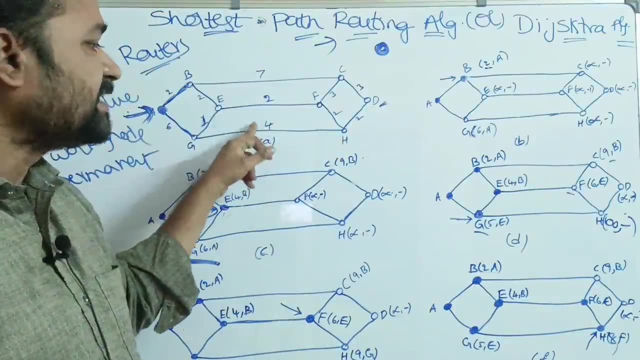 we have to explore G. so what are the neighboring nodes of G? we have only one neighboring node, that is H. so what is the path length here? here, from D to H, the path length is 4. so 5 plus 4 means 9. so infinity comma minus is updated. 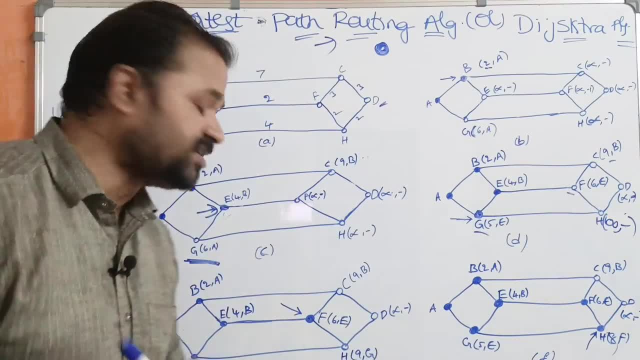 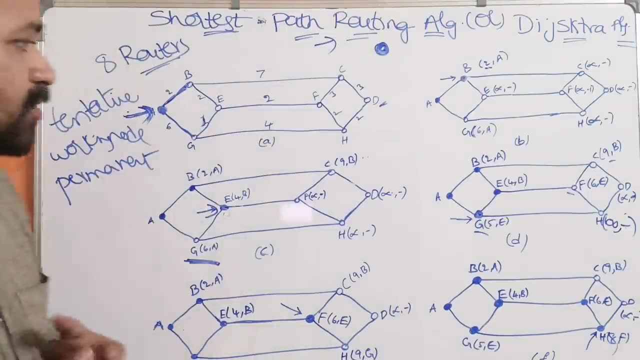 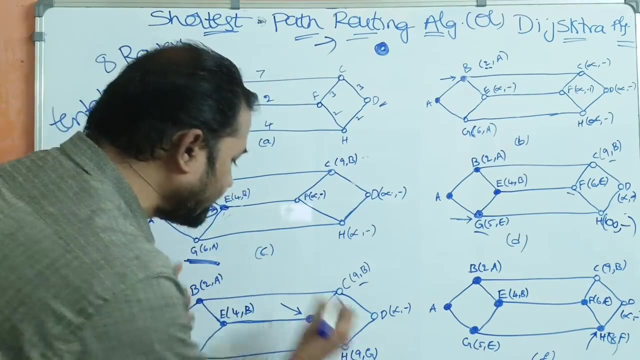 with 9 comma G. so 9 comma G, 9 comma G. so here we have only one neighboring node. so this is the rolling I posso node. so now we need to find out the shortest value. so here this is one tentative node. this is another tentative load and this: 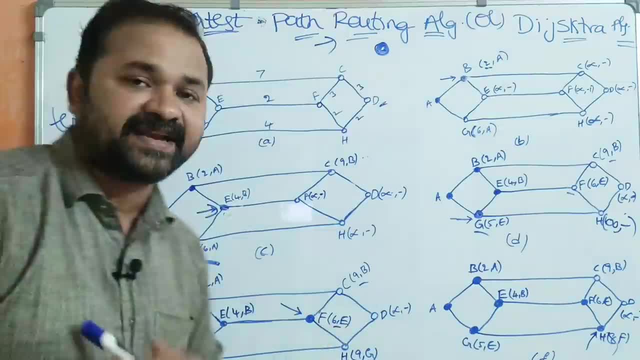 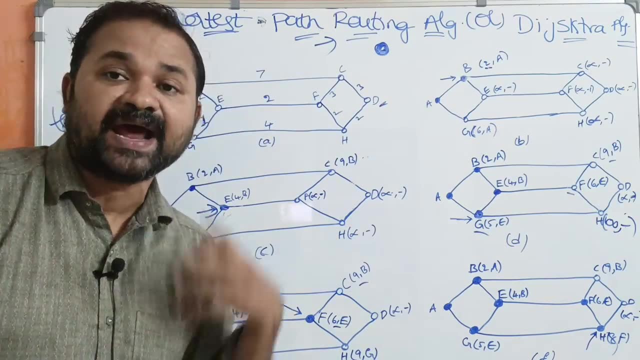 is another tentative node. now, if we find here this is thevised value, so this is the tentative node. so out of nine, six and nine, which is the smaller value, so six is the smaller value. so we have to make this node as the permanent node and current working node. now we need to explore f. 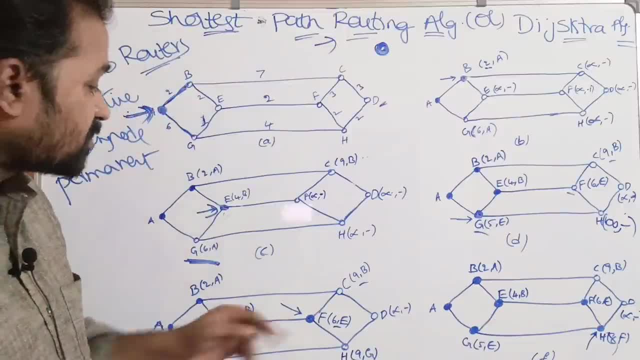 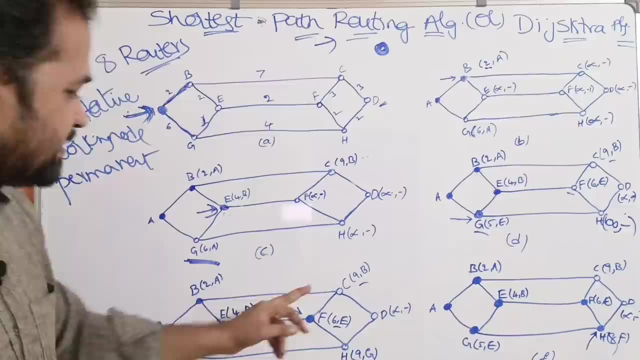 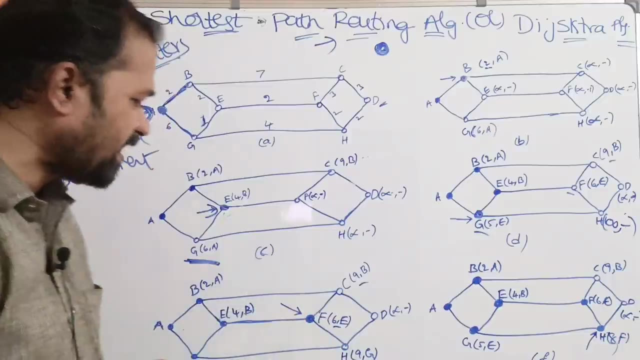 what are the neighboring nodes of f? what are the neighboring nodes of f? we have c, h, we have c and h, so we have two nodes, c and h. so let us find out the cost of h here. uh, so already, uh, the distance of f is calculated. that is six. that is six. now let us find out from: 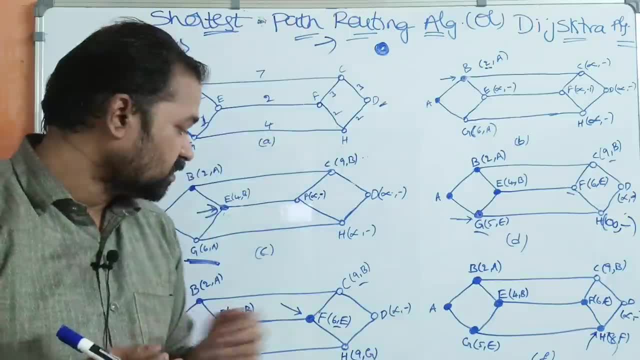 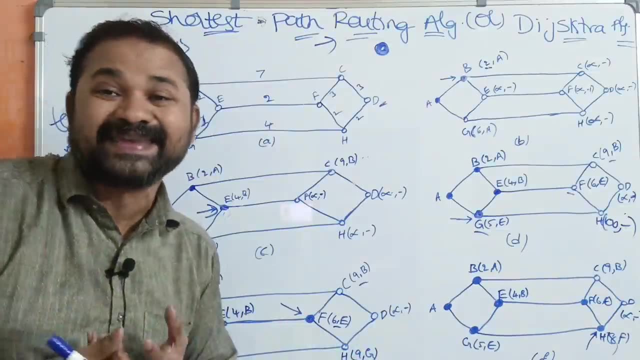 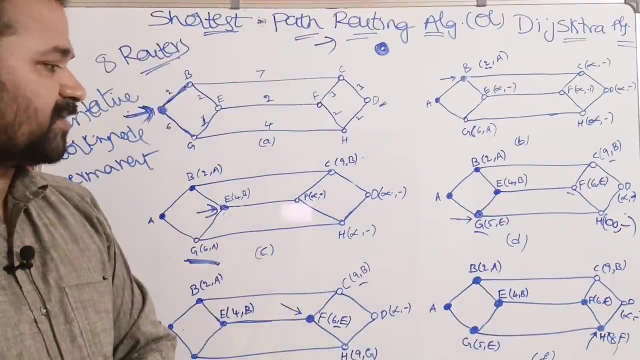 f2g, f2h, f2h. the distance is two, so six plus two. six plus two means eight. so previously the cost is nine, but now we got eight. so nine comma g is updated with eight comma f, eight comma f, eight comma f. so next, out of nine, eight, which is the smaller value, eight is the smaller. 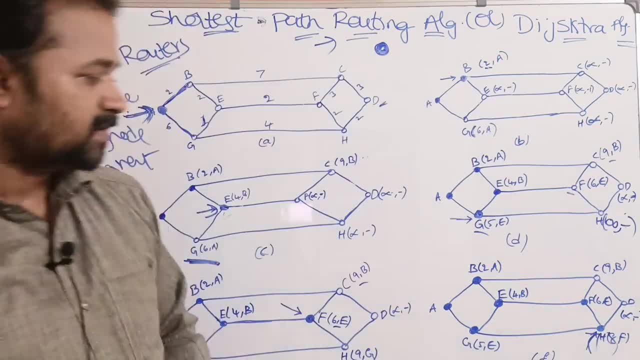 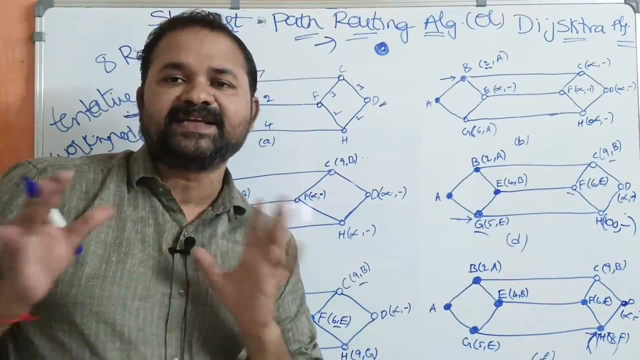 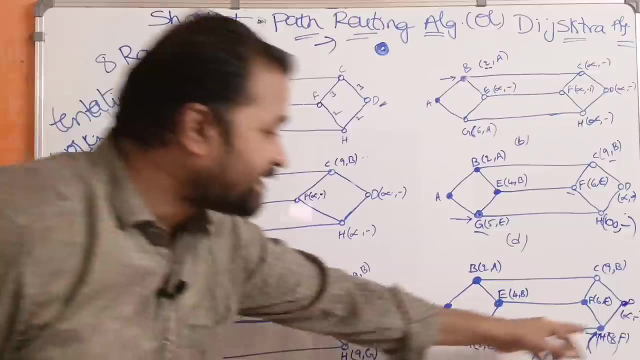 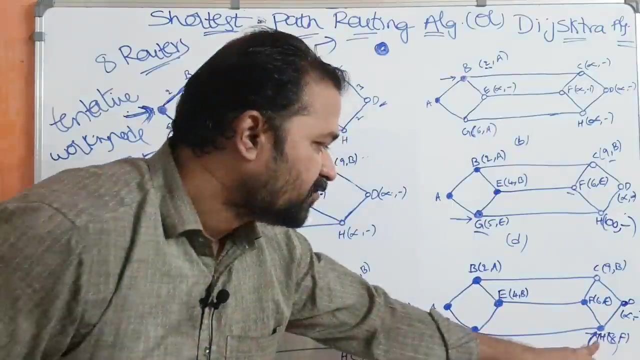 value. so now we have to explore this node. so from h directly we can go to the d. so this is the path here. so now let us write the path here. so here, what is the destination router? d is the destination router. so we are traversing to d. from which node? from which node? h, h. next we are traversing to h. 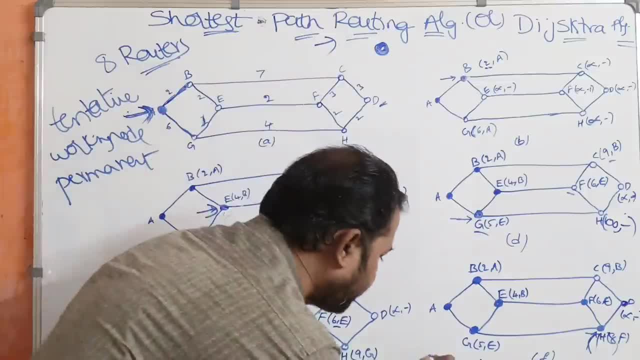 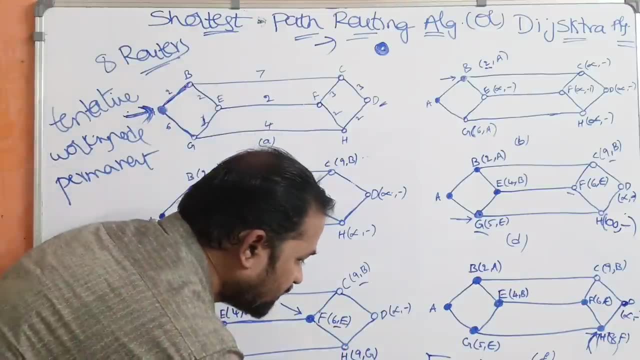 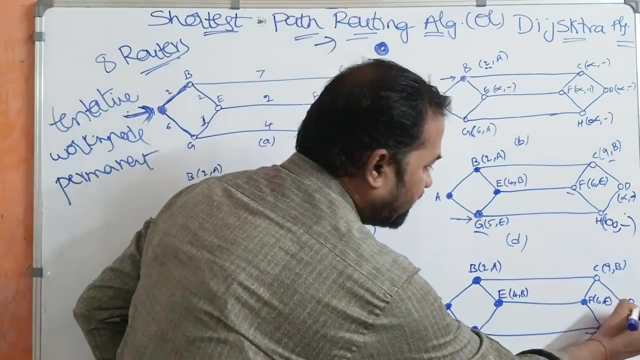 from which node h, 8 comma, f, f, f. so let us see f. we are traversing to f. from which node e, e? yeah, it is not visible. let us write a little bit upper side. so here, what is the destination node? d is the destination node. 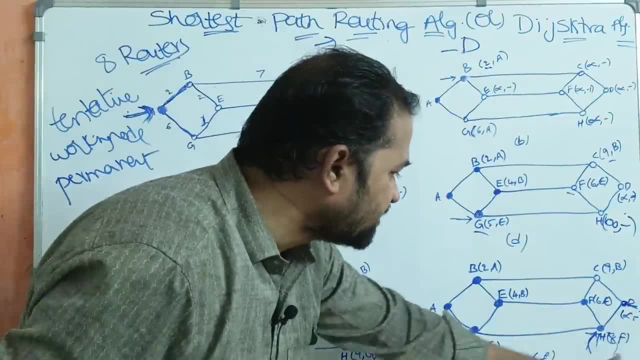 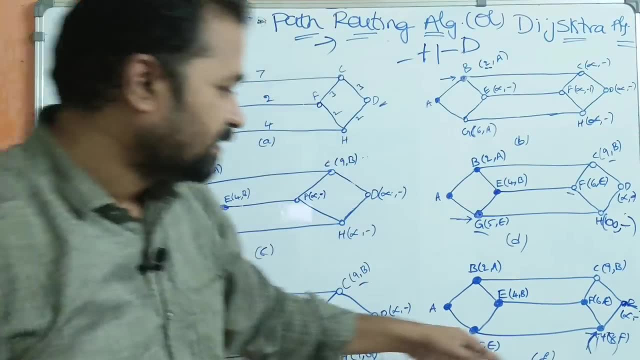 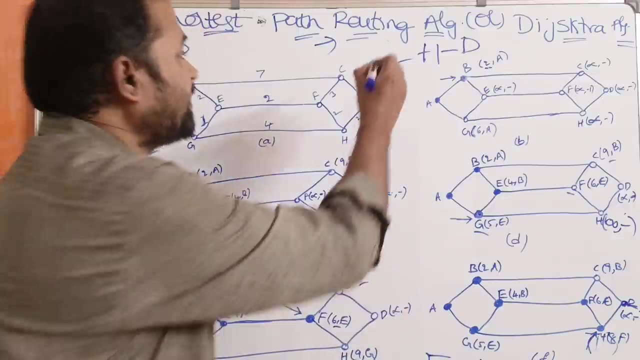 d is the destination router, so d. we are traversing to d from h. this h, so h. let us find out the shortest path. next d: h. we are traversing to h, from which node h, 8 comma, f, so f, f. so let us see f. we are traversing to f from. 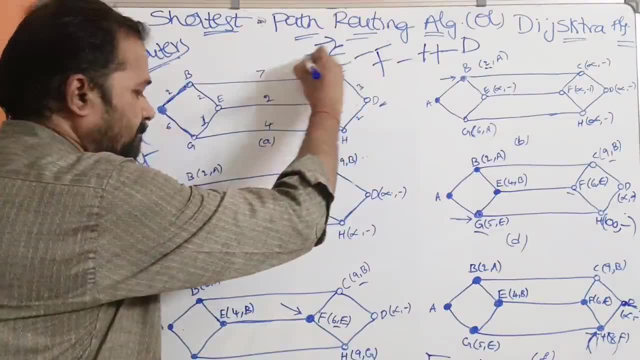 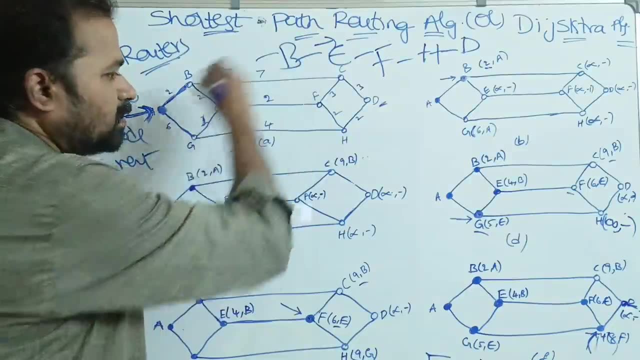 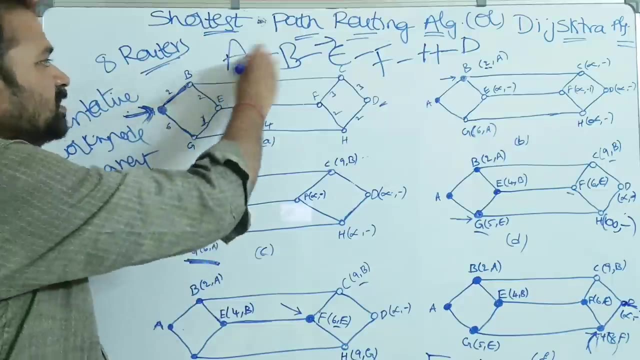 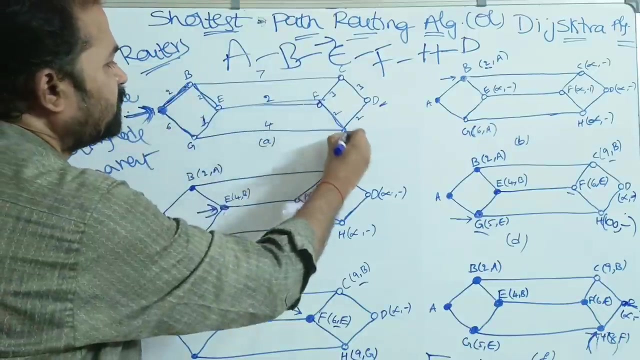 which current the working node e. so e, next e we are traversing to e. from which node which router? b. next we are traversing to b, from which node a. so this is the shortest path: a to b, next b to e, next e to f, f to h, h to d. so what is the cost here? 2 plus 2 plus. 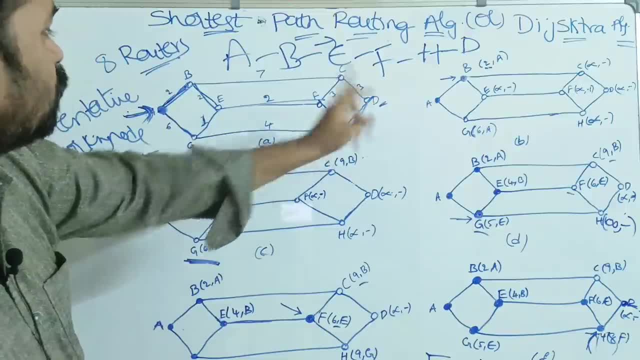 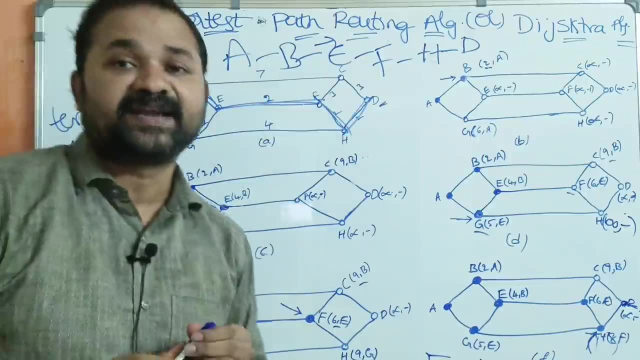 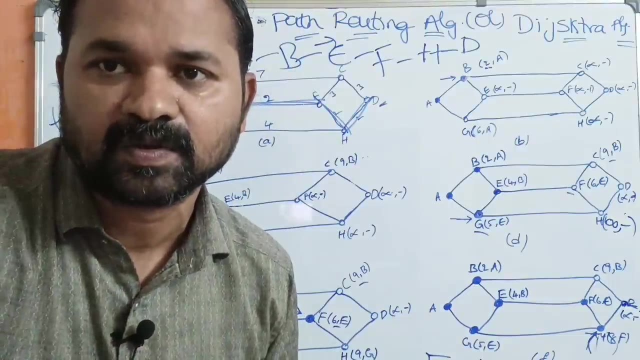